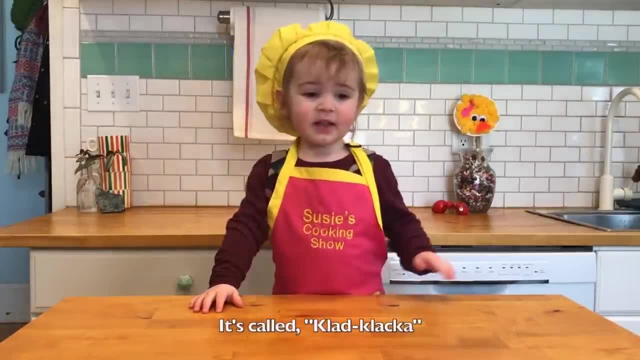 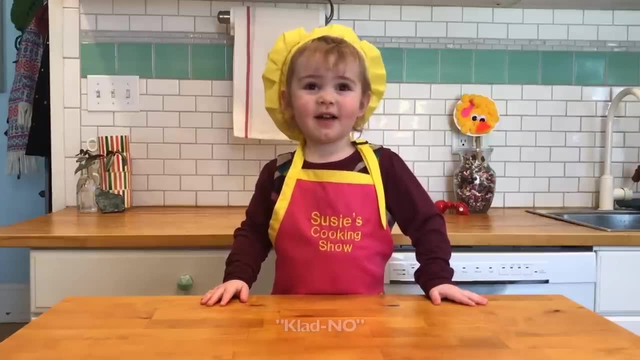 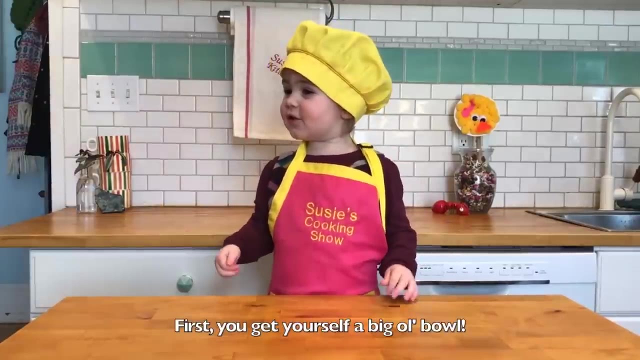 It's Swedish To make this chef. it's called a claw, clarka Claw, clarka Claw, clarka Claw. No, Okay, ready, Let's get started. First you get yourself a bigger bowl. Oh, you want a bigger bowl, Suzy. 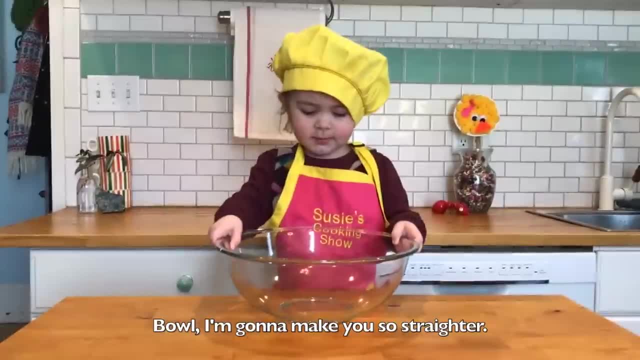 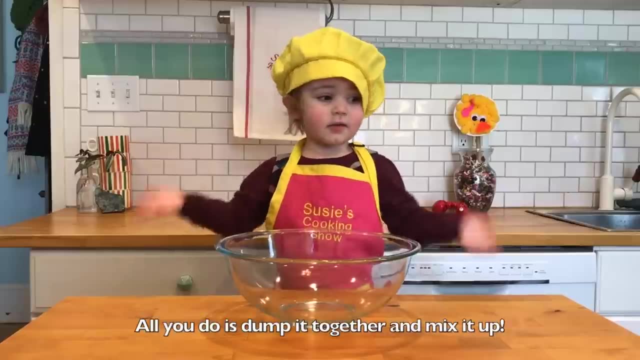 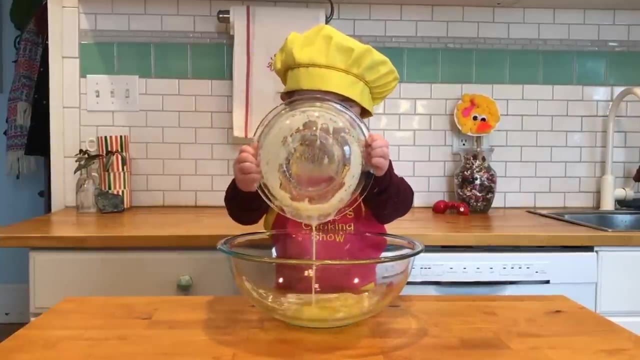 I love my bowl Bowl. I'm going to make you so stuttered. This recipe is for grateful kids. All you do is dump it together and mix it up Half a cup of melted butter. Next, add the sugar. I need you to help me, though. 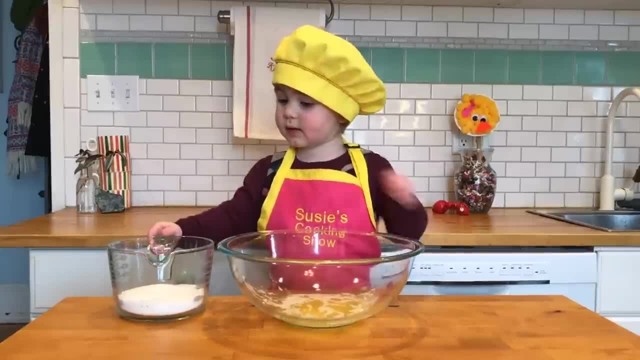 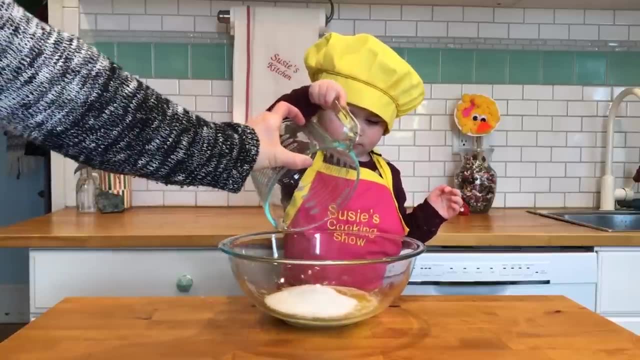 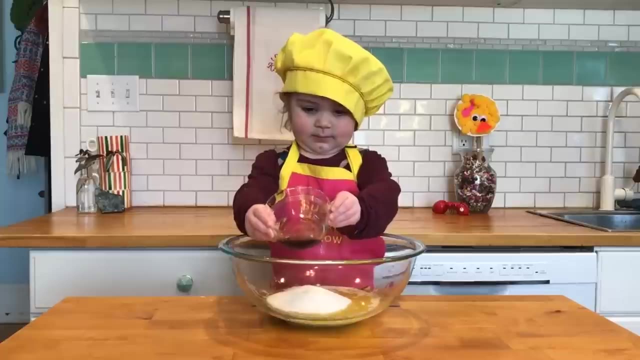 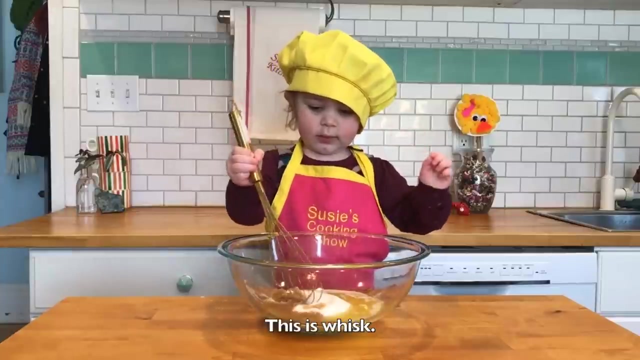 You can help me. you can help me, Help me, Help me. You can help me, help me, help me. One tablespoon of vanilla. This is vanilla. Vanilla, Vanilla, Vanilla. This is whiskey. One half a cup of flour. 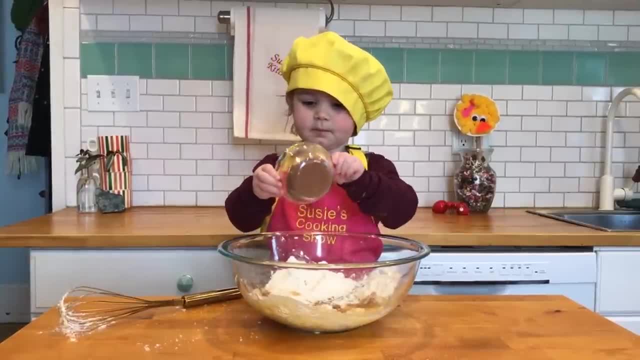 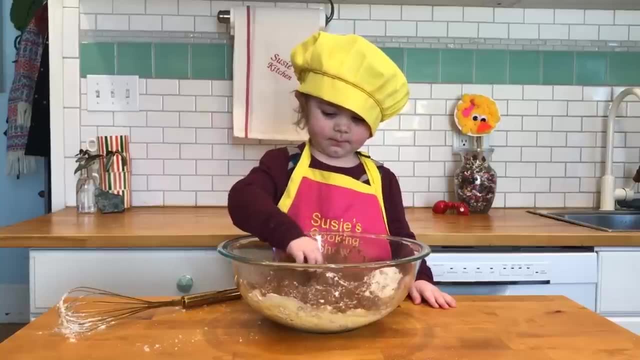 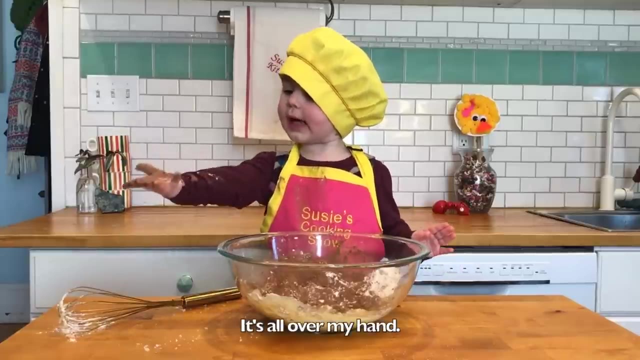 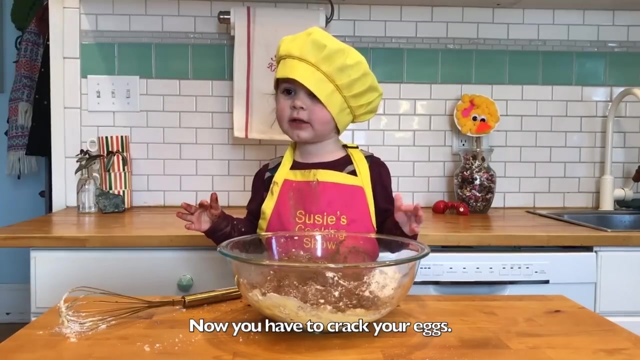 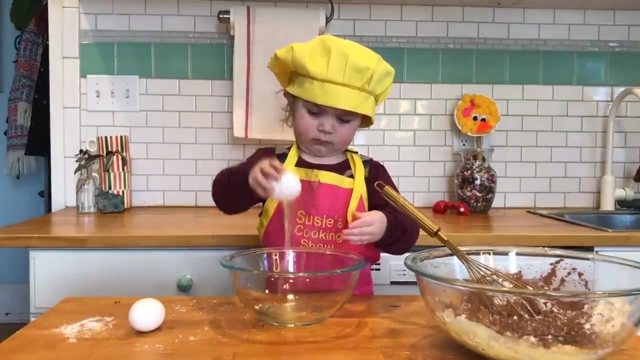 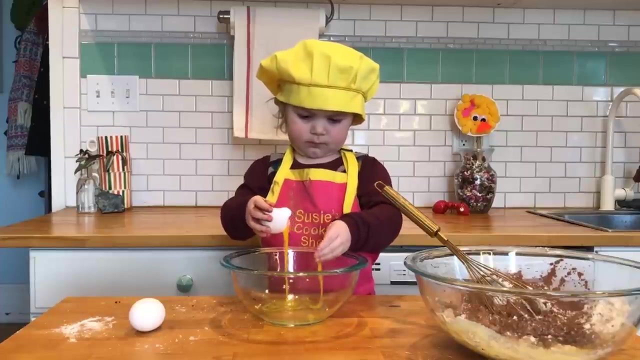 This one is cocoa powder, Mmm. Chocolate. It's good, Mmm, It's all in one hand. Wipe it off, wipe it off, Thank you, Thank you. Now you have to crack your eggs. Wipe it off, wipe it off. 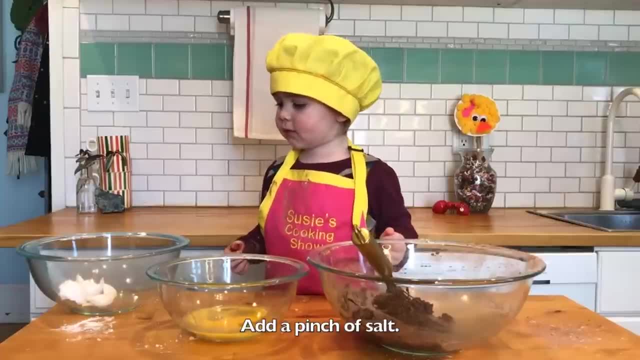 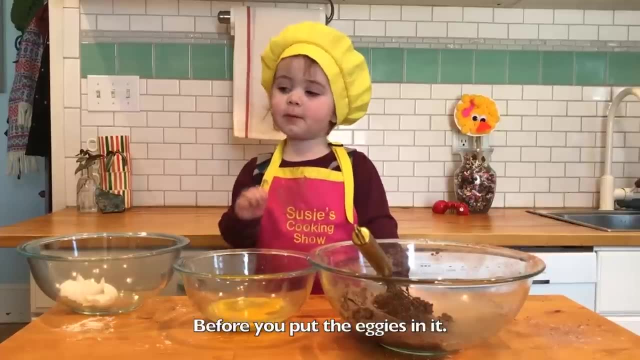 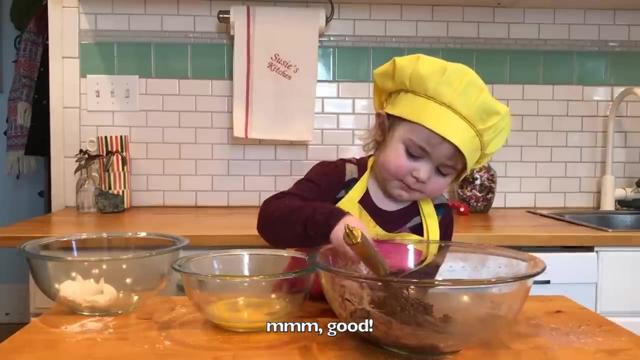 Make sure you put it on your own. I want a piece of salt When you want to taste it. that's how you're gonna do it Before you put the egg in it: Mmm, Mmm, good, Mmm. 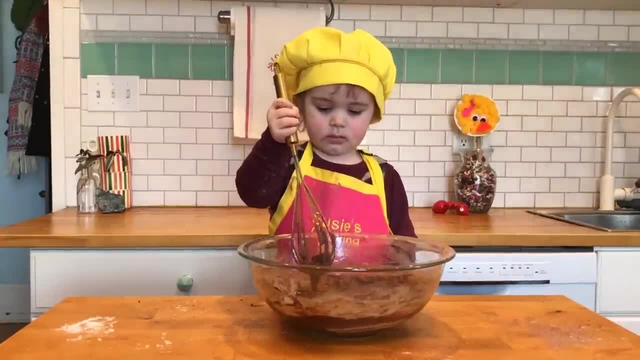 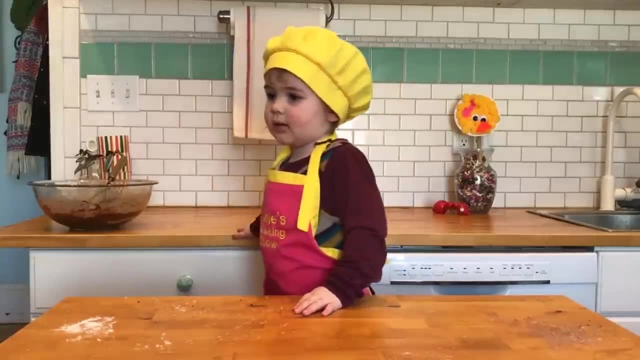 I'm sad because I want to eat that one, But I can't because it has a lot of eggs in it. Now you're gonna prepare your pan. My mom bought me the pan, so I need some more of that. Here's another cool tip.